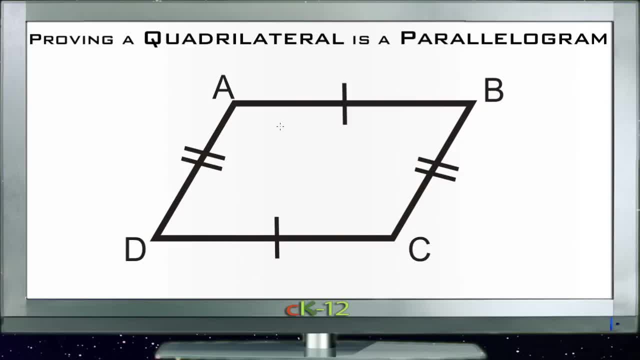 we can use all that other information that we know about parallelograms. Really, what we're going to do is use the theorems that we identified as being parts of a parallelogram in reverse, and then we can use them to describe whether or not a figure is a parallelogram. 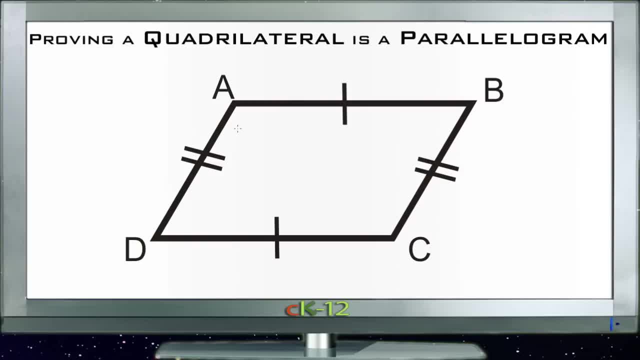 So first of all we're going to talk about the opposite sides theorem. Recall that if a figure is a parallelogram, then the opposite sides are congruent. So that's the parallelogram As we see with this figure marked here. side AB across the top is congruent to DC across. 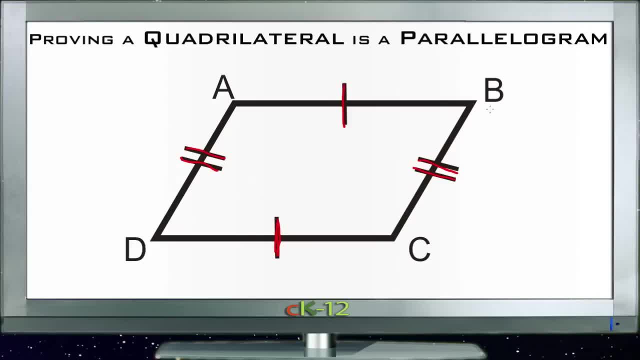 the bottom and AD down the left is congruent to BC down the right. If you know that both pairs of the opposite sides of the quadrilateral are congruent as they are here, then you know that the figure is a parallelogram, So that's the converse of the opposite sides. 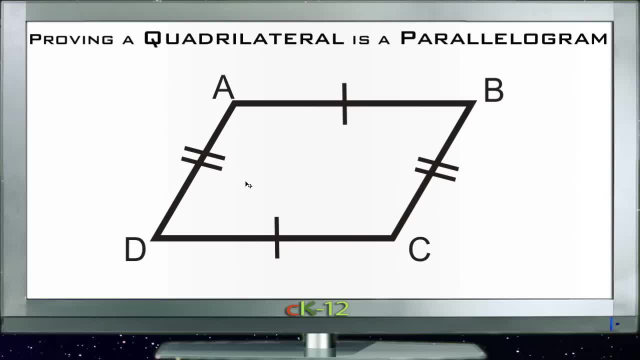 theorem. Now, similarly, like we had the opposite sides theorem, we had the opposite angles theorem, and we can use it as well. If we knew, for instance, that angle A here was congruent to angle C and that angle D was congruent to angle B, then that also can be used to. 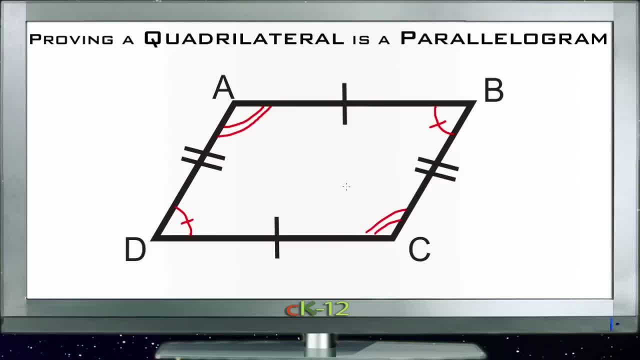 show that the figure is a parallelogram. That's the converse of the opposite angles theorem. Then we have the parallelogram diagonals. If you recall, the diagonals of a parallelogram, say from D to B here, or from A to C here, are congruent to the opposite sides of the 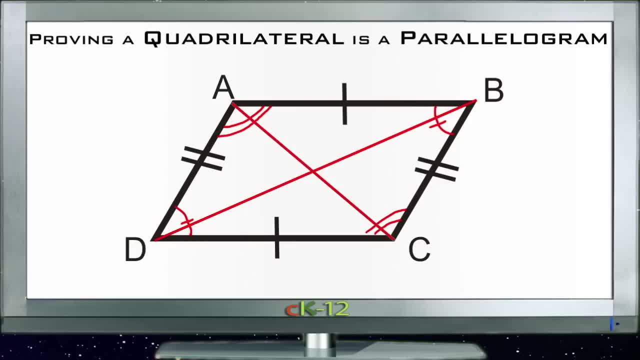 quadrilateral, You can see that the diagonals of a parallelogram bisect each other. So if you have a figure and you know that the diagonals of that figure bisect each other, so that this section from the center point to B is equal to the center point to D, We'll call 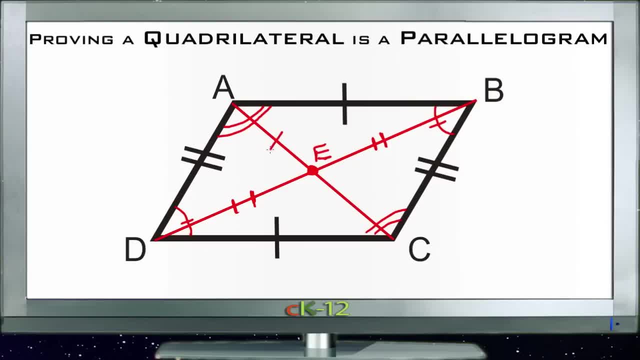 this E out here. If this from A to E is congruent to E to C, then you also know that the figure is a parallelogram. Finally, if a quadrilateral has one set of parallelograms, it has two set of parallelograms. 2 of A's, 0 of Z, 0 of R, 0 of A and 2 of G. So that's been able to чув that the leich of this idea, which looks usually n legal diagram of a parallelogram and its apparent. 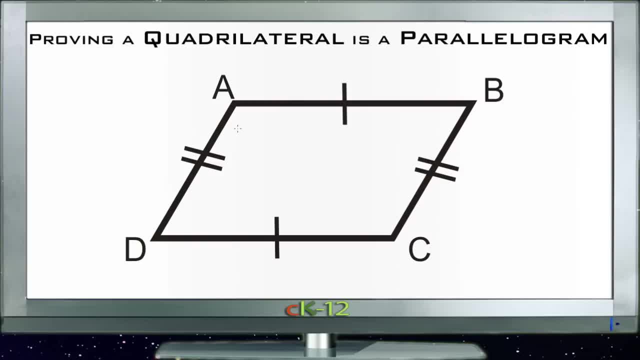 So first of all we're going to talk about the opposite sides theorem. Recall that if a figure is a parallelogram, then the opposite sides are congruent. So that's the parallelogram As we see with this figure marked here. side AB across the top is congruent to DC across. 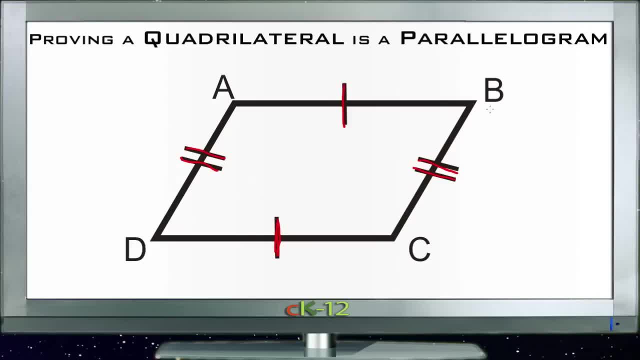 the bottom and AD down the left is congruent to BC down the right. If you know that both pairs of the opposite sides of the quadrilateral are congruent as they are here, then you know that the figure is a parallelogram, So that's the converse of the opposite sides. 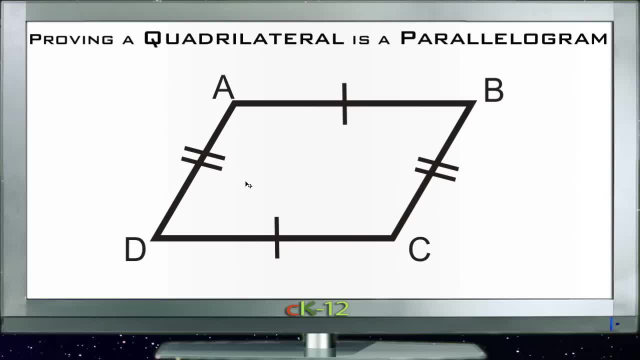 theorem. Now, similarly, like we had the opposite sides theorem, we had the opposite angles theorem, and we can use it as well. If we knew, for instance, that angle A here was congruent to angle C and that angle D was congruent to angle B, then that also can be used to. 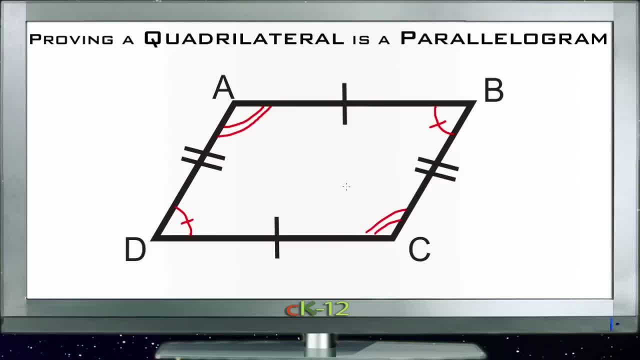 show that the figure is a parallelogram. That's the converse of the opposite angles theorem. Then we have the parallelogram diagonals. If you recall, the diagonals of a parallelogram, say from D to B here, or from A to C here, are congruent to the opposite sides of the 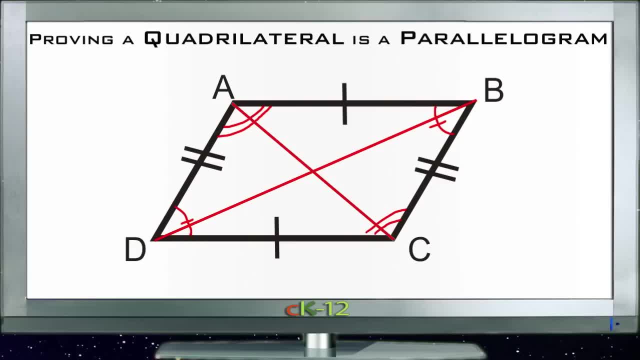 quadrilateral. So if you have a figure and you know that the diagonals of that figure bisect each other so that this section from the center point to B is equal to the center point to D, we'll call this E out here- and that from A to E is congruent to E to C. then 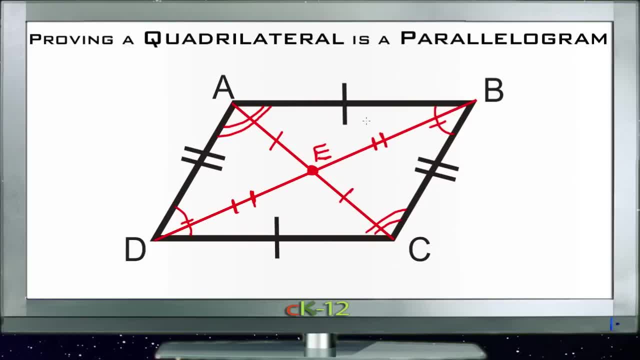 you also know that the figure is a parallelogram. And finally, if a quadrilateral has one set of parallel sides that are congruent, in other words, if we know that, for instance, side AB here side AB is parallel to side DC and that those two sides are the same, then we 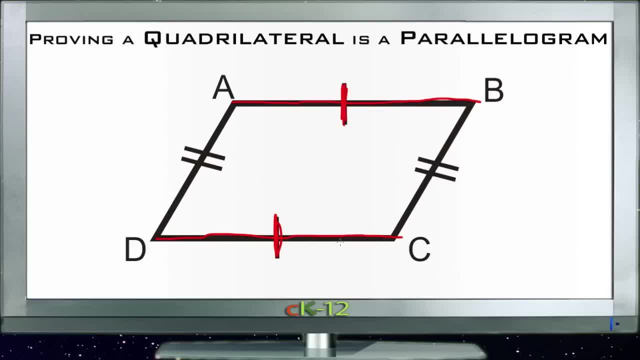 know that the figure is a parallelogram. These two sides can't be parallel to each other and be identical without these two sides over here being the same thing. So either we can show that the two pairs of sides are the same as each other or we can show that one pair.